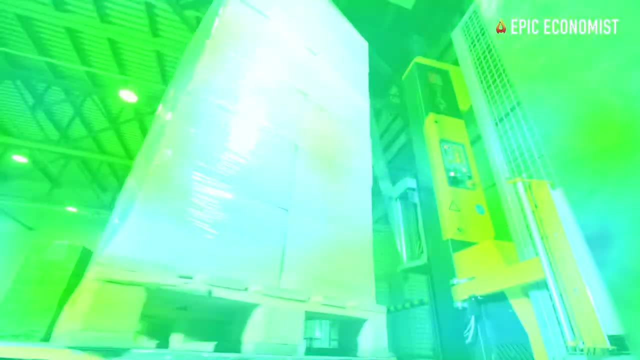 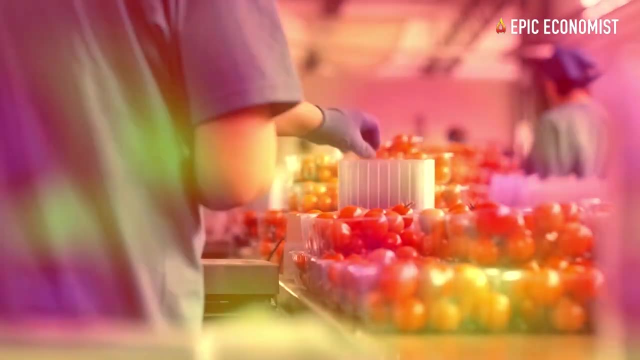 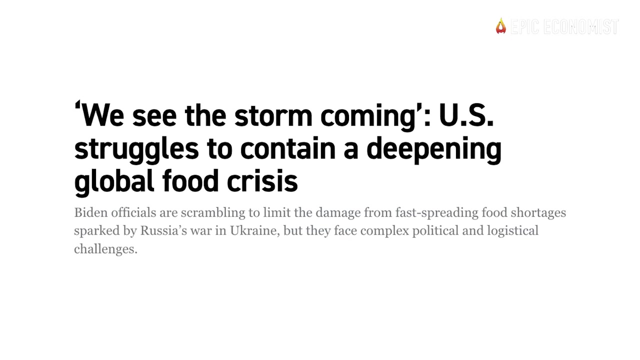 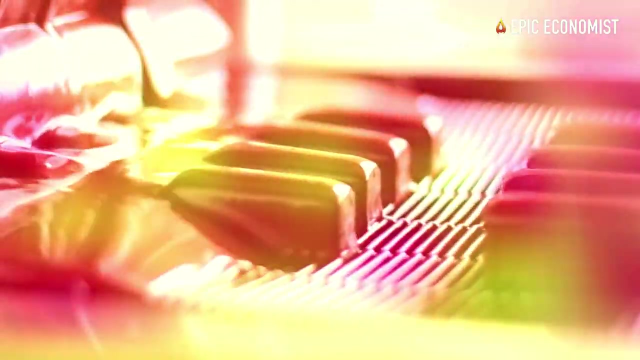 A global food shortage of catastrophic proportions has already begun, and things are only going to get worse. from this point on, The information we're about to expose might be hard to digest, but we would like to encourage you to share this message with everyone you care for, so that people can. 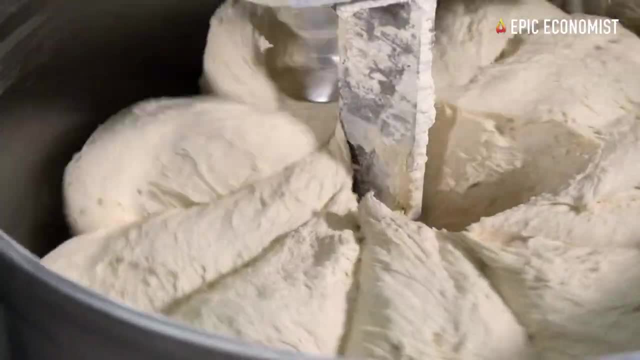 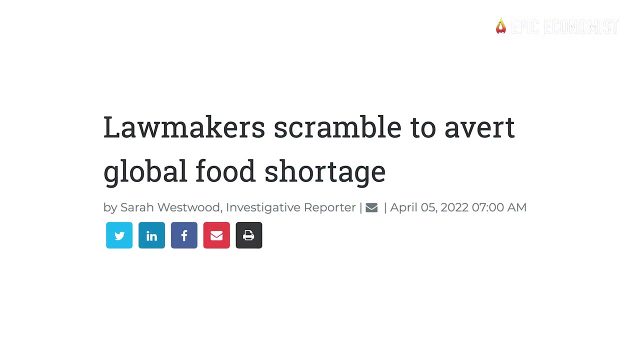 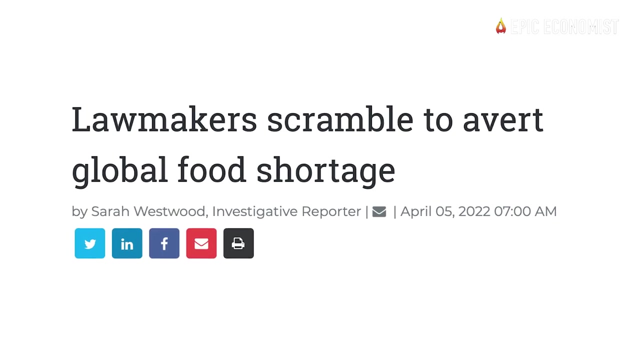 prepare for what is coming. Everybody deserves to know what is truly going on, and they deserve an opportunity to get ready before this crisis gets out of control. The pace at which things are changing all over the world right now is extremely alarming, but somehow many people still. 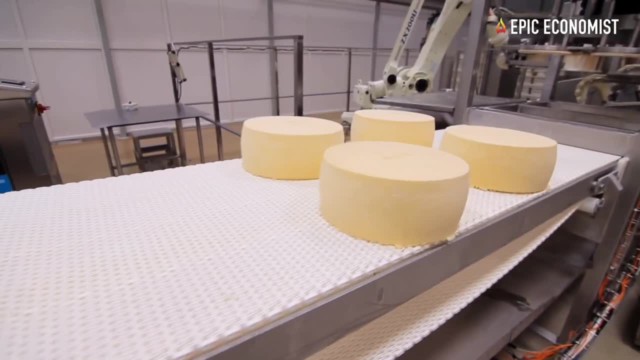 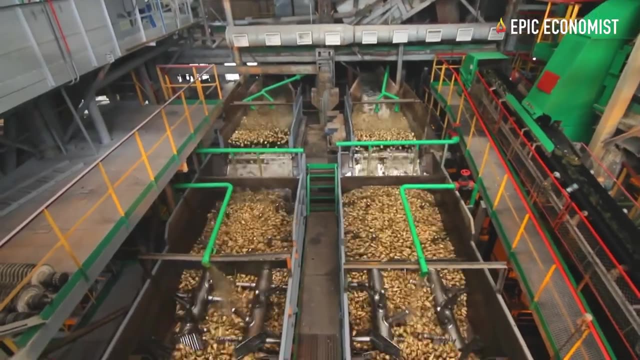 believe life will just continue to carry on as it normally does. Sadly, the truth that we're about to expose might be hard to digest, but we would like to encourage you to that. a very real planetary emergency is unfolding right before our eyes, and we must act before it's. 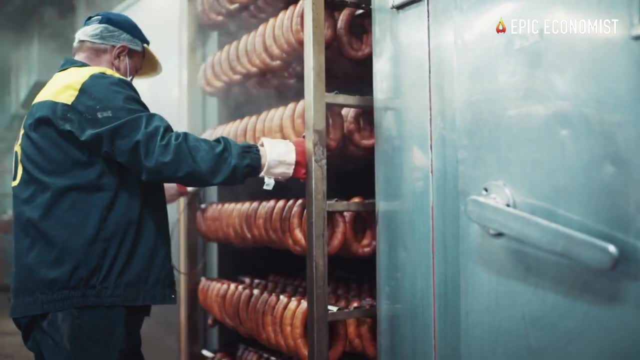 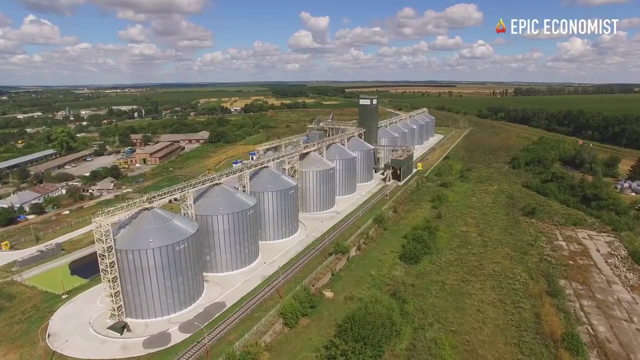 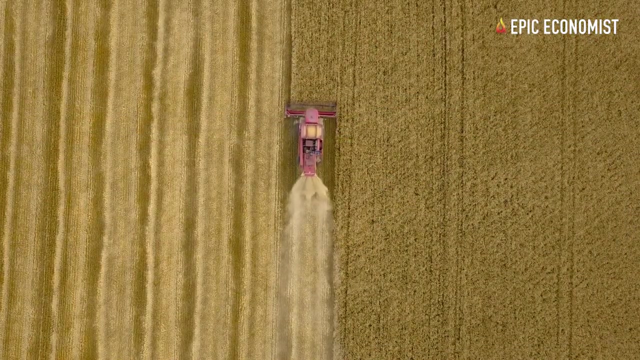 too late. In today's video, we have compiled facts that reveal the humongous proportions of the global food crisis, But before checking this list, don't forget to leave a thumbs up. please subscribe to our channel and turn on the bell so you can keep updated. 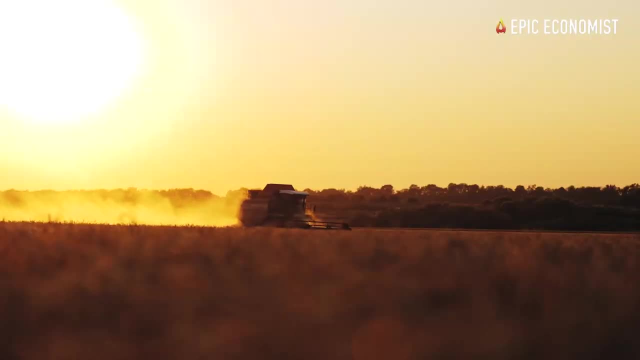 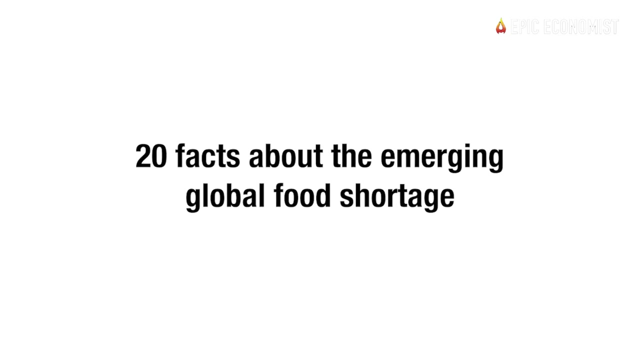 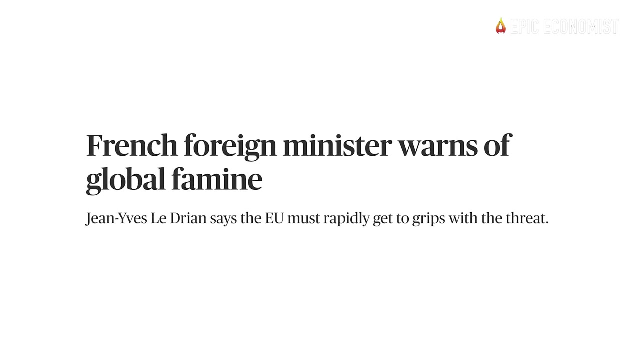 with our latest notifications. Here are 20 facts about the emerging global food shortage that should chill you to the core. Number one: one of France's most important government officials is warning the public to brace themselves for widespread food shortages In a recent statement. 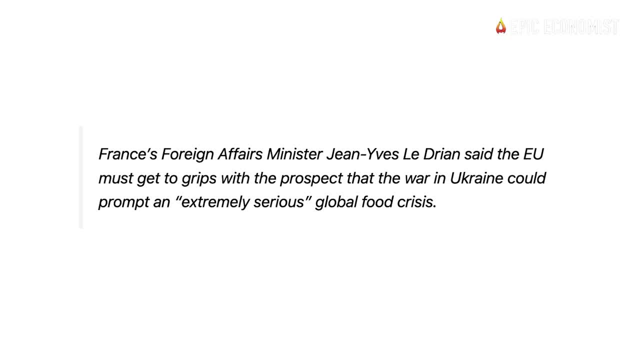 France's foreign affairs minister, Jean-Yves Le Drian, said that the world must, in turn, get to grips with the fact that the conflict in Ukraine is prompting an extremely serious global food crisis Number two. the President of the United States has openly 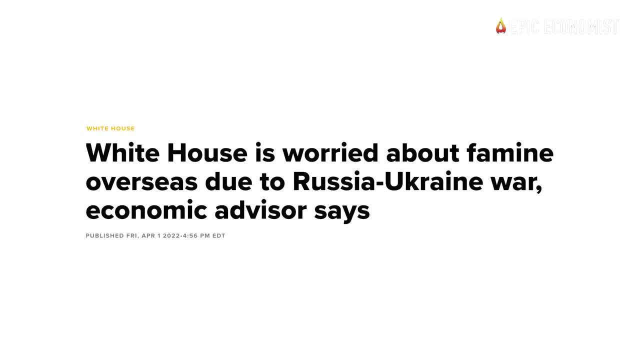 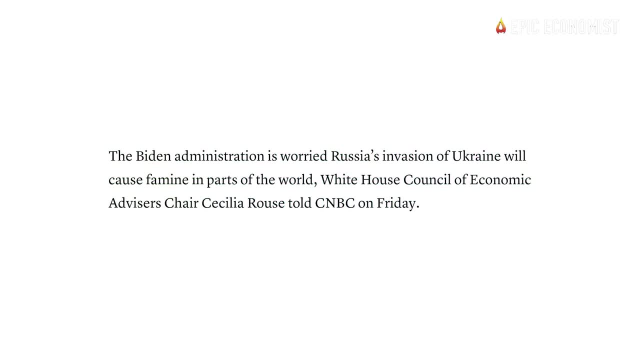 admitted that extensive food shortages are going to be real and his officials are concerned about the prospect of a hunger crisis. The Biden administration is worried. Russia's invasion of Ukraine will cause famine in several parts of the world. Russia's invasion of Ukraine will cause famine in several parts of the world. Russia's invasion of Ukraine will cause famine in several parts of the world.